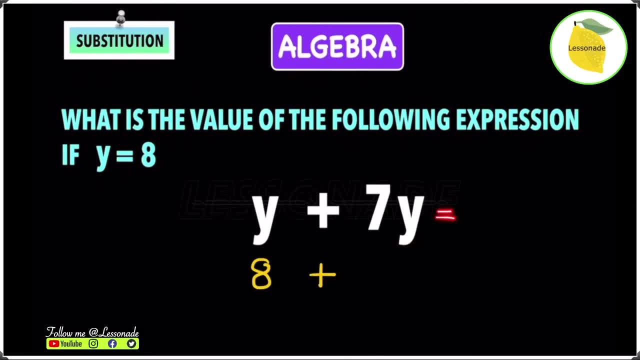 For the seven y. however, seven y is the same as seven times y. Because it's the same as seven times y, when you replace this y, you're going to get seven times eight. So whenever you have a multiplication such as seven y, you're always meant to expand it when you substitute Otherwise. 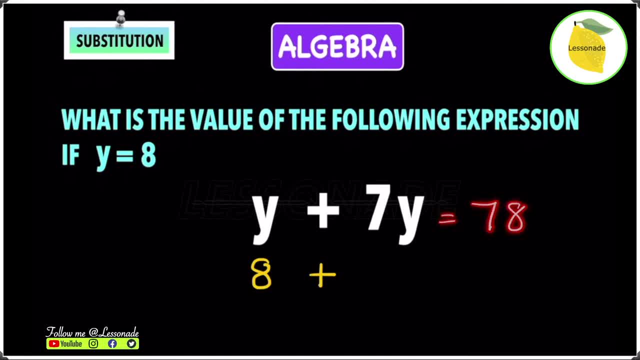 if you don't expand it, you're going to get a multiplication. you're going to be left with 78, which is not right. Instead, you have to expand it to 7 times y and then you can substitute this y. So we have 7 times y, and when you substitute this y, 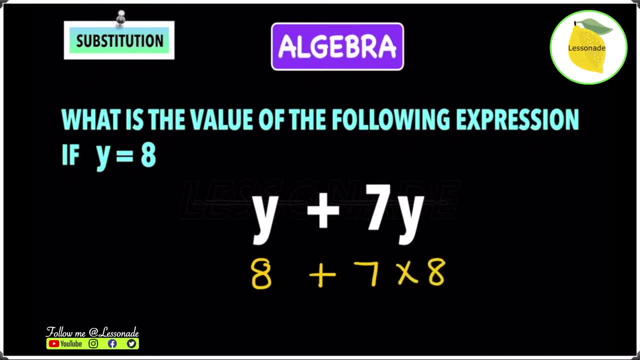 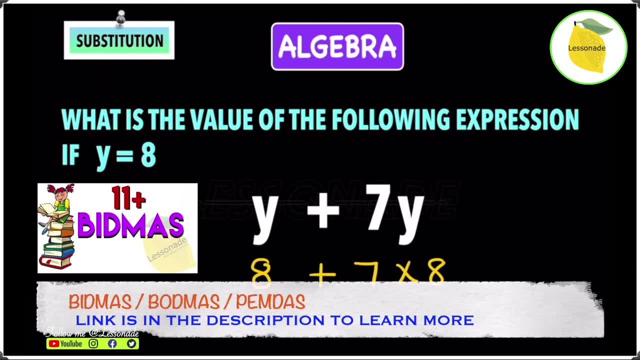 basically going to get 7 times 8.. The next thing: we have to work this question out and we have 8 plus 7 times 8.. Things to remember: in this case we have to use bitmass If you guys want. 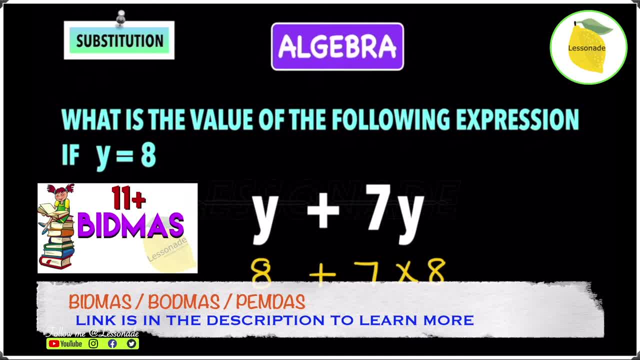 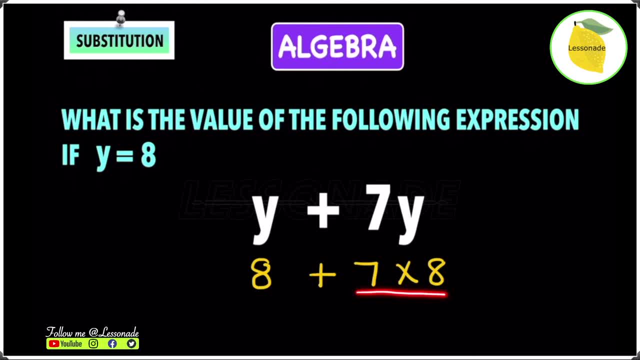 to know more about bitmass. I've got a video on bitmass. Go check the video out. The link is in the description below. So we have 8 plus 7 times 8. You have to first do 7 times 8, because 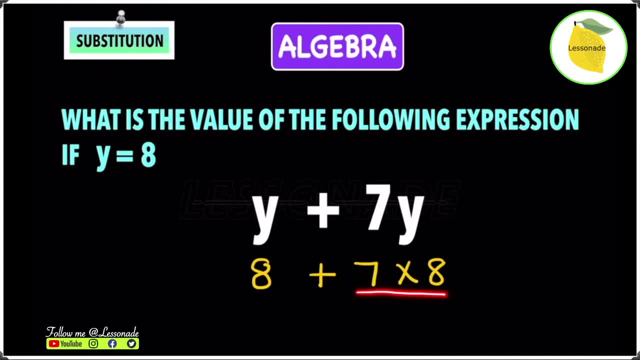 multiplication is higher up than addition in bitmass or in the order of operation. So 7 times 8 will give you 56, and then you have to add this 8, and then 8 plus 56 will give you an answer of. 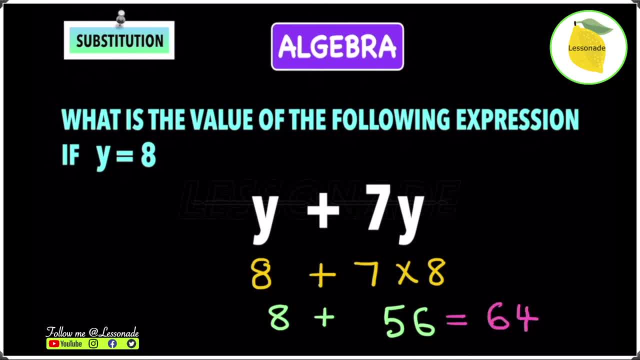 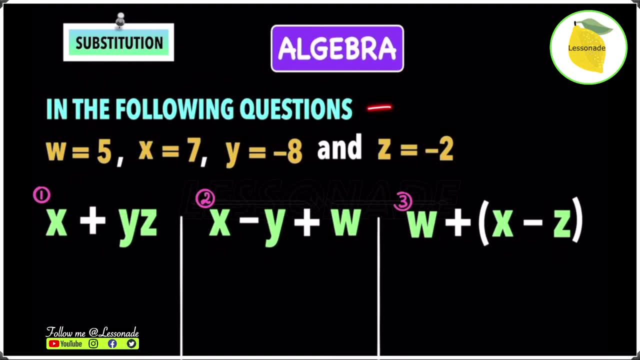 64. So that means your answer to this question is 8 plus 7 times 8, and then you have to add this to this question is 64.. And let's have a look at another example in algebra substitution And in this example it says in the following questions: w equals 5, x equals 7, y equals minus 8, and z. 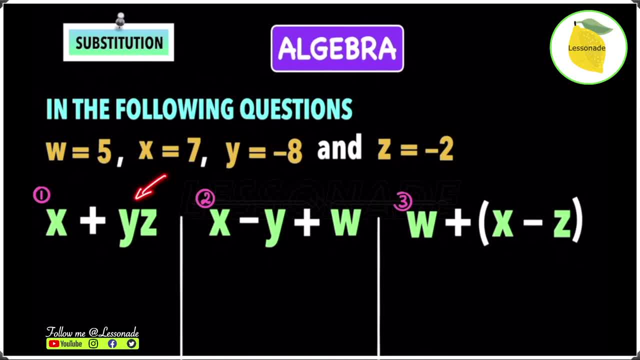 equals minus 2.. And let's start with the first example, which is x plus yz. So we know that the x is obviously x equals 7, which means we need to substitute a 7 for this x, So we can write. 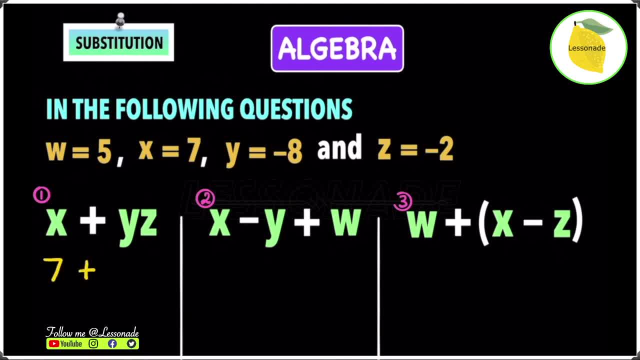 the x. The next thing we have to do is substitute for this yz And, as we all know, yz is the same as y times z. So we know that yz is the same as y times z, And we know that y is minus 8.. And we 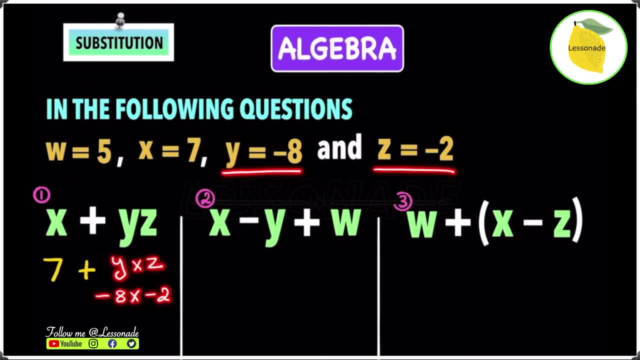 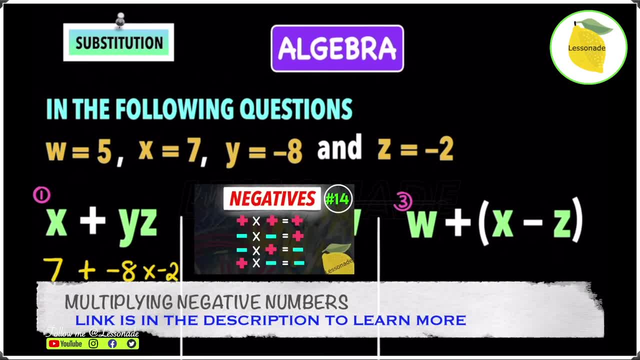 also know that z is minus 2.. So we're going to do minus 8 times minus 2.. So write that down: minus 8 times minus 2.. Now we have 7 plus minus 8 times minus 2.. 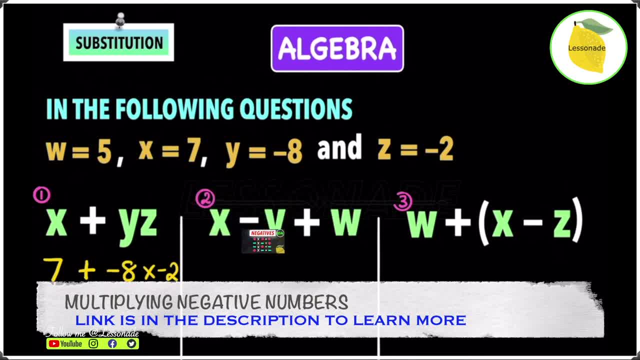 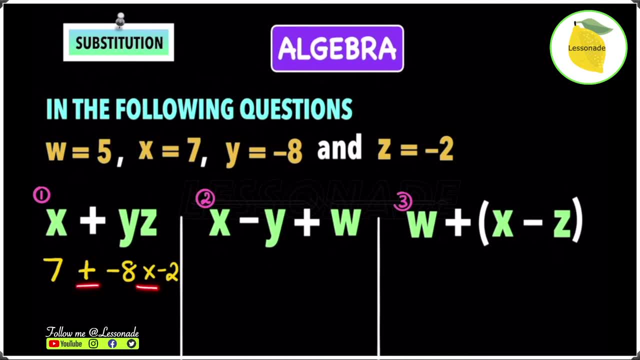 This question might look a bit confusing at the start, but as you go through it it will be much more easier. So we know that we have plus and multiplication, We have addition and multiplication, And according to bit mass or the order of operation, multiplication is higher up, So we do. 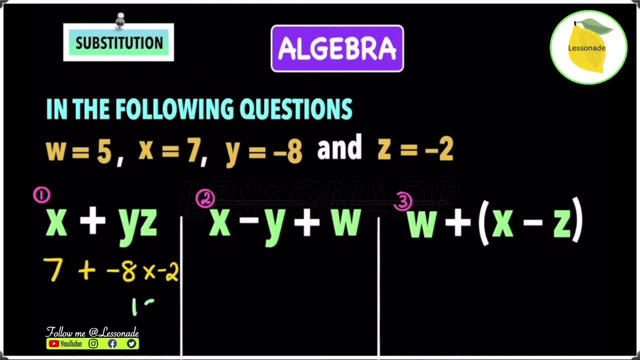 multiplication first. So minus 8 times minus 2,, 16.. And the next thing: we have to add this to the 7. 7 plus 16 will give you an answer of 23,, which means our answer is 23.. Let's have a look at. 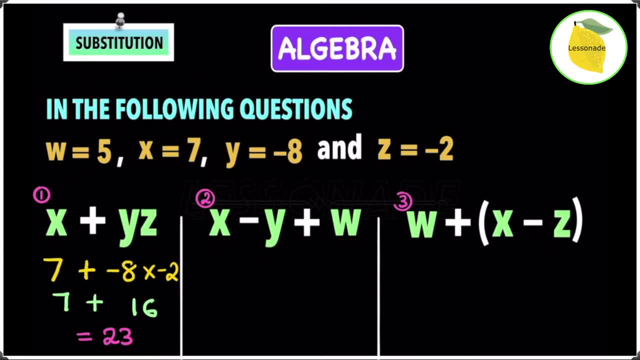 such as x minus y plus w, x minus y plus w. We know that x is 7.. So substitute the 7 for the x, And we know that the y is minus 8.. So write down the minus 8 as well. So once you've done that, 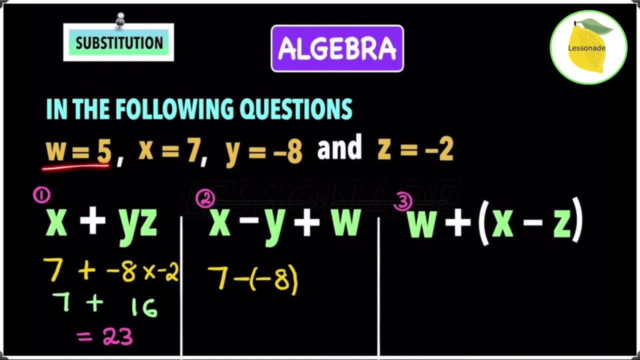 the next thing we have to do is to add the w, which is 5.. So we have to do plus 5.. And now this question might look a bit difficult, because we're doing 7 minus minus 8 plus 5.. 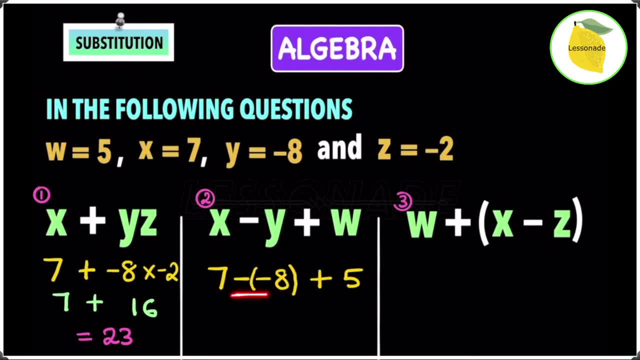 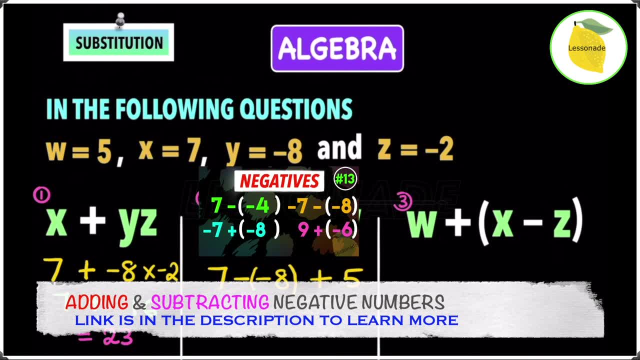 And, as you guys could see, we have two minuses next to each other. Because we have two minuses next to each other, we have to do this a bit differently. If you guys want to know more about subtracting and adding negative numbers, I've got a video on that as well. The link is in the 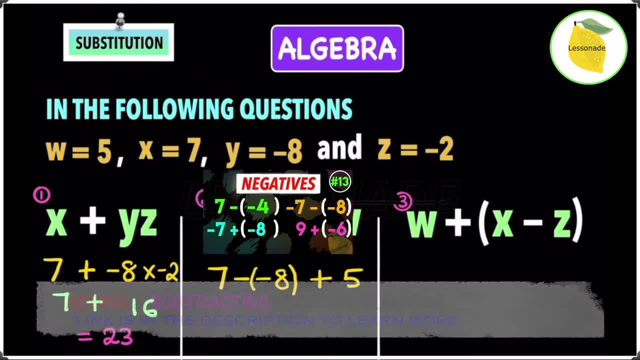 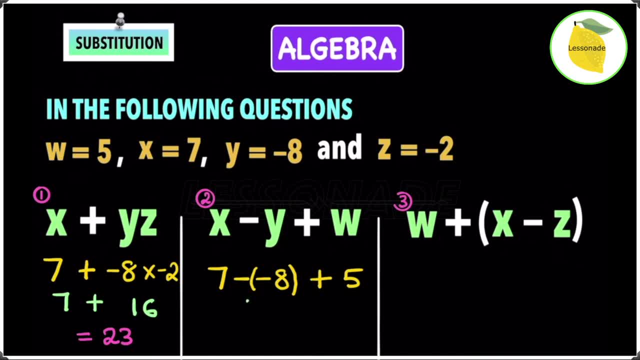 description below. So go check that out. And whenever you have two of the same signs next to each other, such as plus or minus next to each other, then you always do addition. So basically add the 5 at the end. So now this question looks much more simpler. So 7 plus 8 will be 15.. 15 plus. 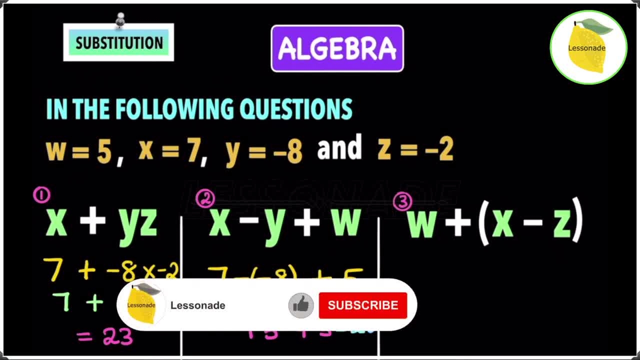 5 will give you an answer of 20.. So let's move on to our final example, which is w plus brackets, x minus z. So in this example, as you guys could see, we have brackets. So let's start by substituting. 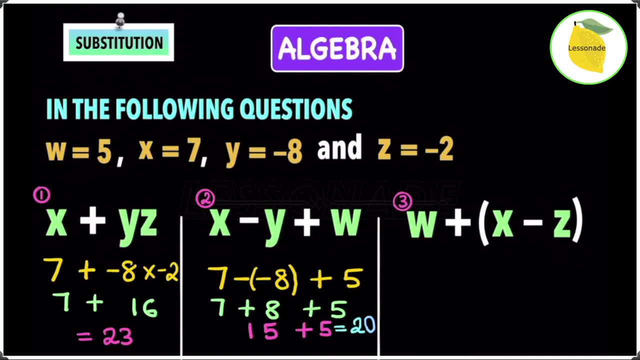 this w first. The w is 5.. So write a 5 underneath. Next thing, we're going to add this to the brackets, which are x minus z, And we know that x is obviously 7.. So that means write a 7 underneath the x, And then the z is going to be.